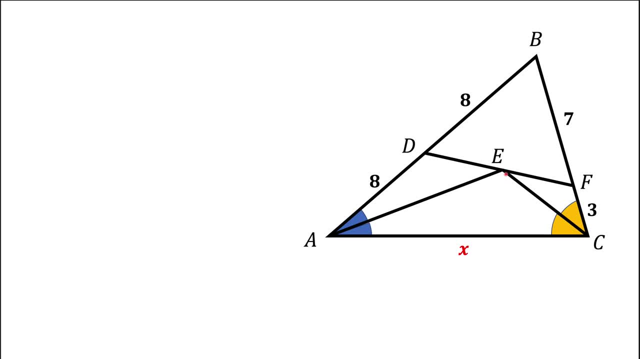 D and F Goes through point E. So how are we going to do this? Well, first let's do a little bit of looking. And one thing: we noticed that E is the point of intersection of two angled bisectors, And we know from geometry that in a triangle all three angled bisectors intersect at the same point. 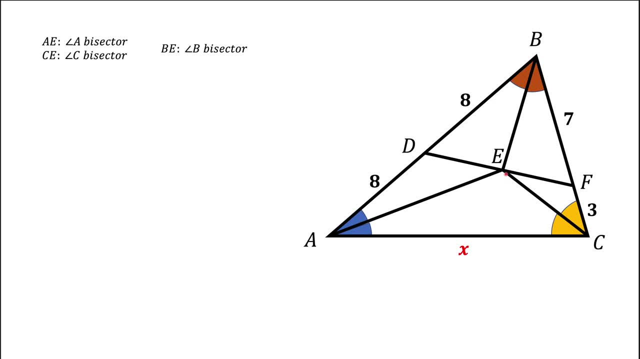 So, which means that BE is going to be an angled bisector as well. The other thing you know about this point E is that is the center of a circle that is inscribed in this triangle ABC. So inscribed circle is a circle that doesn't come out in any part outside of the triangle ABC. 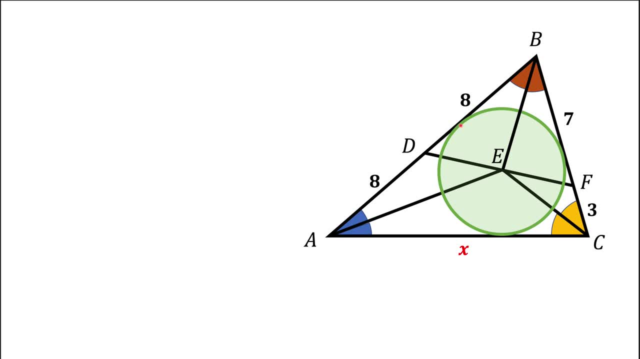 And that's the largest circle you can put inside of the triangle ABC. The sides AB, BC and AC are tangent lines to this circle, which means that there is only one, and only one point that this circle shares with line AB. Let's call it H1.. 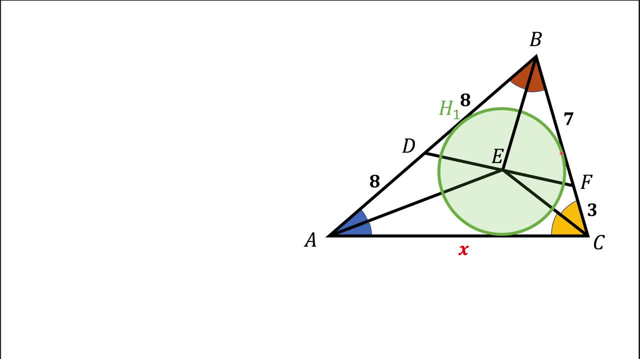 There is one point that a circle shares with line BC. Let's call it H2.. And a point which the circle shares Shares with line AC. We call it H3. Now, what we're going to do next is we're going to connect those H1, H2, and H3. 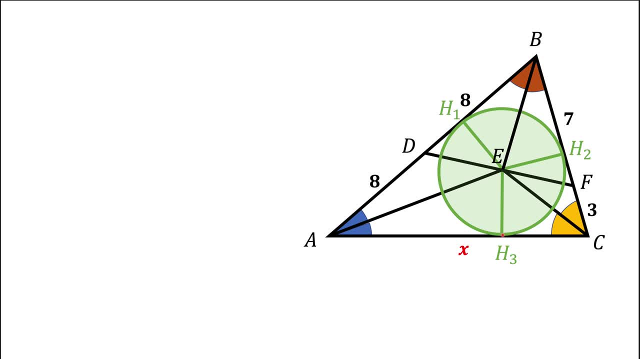 Use the center of a circle E, So all these three segments have the same length, equal to the radius of the circle. There is another property that relates the circle and a tangent line, And that is that the tangent line, like AB, and this radius EH1, are at 90 degrees to each other. 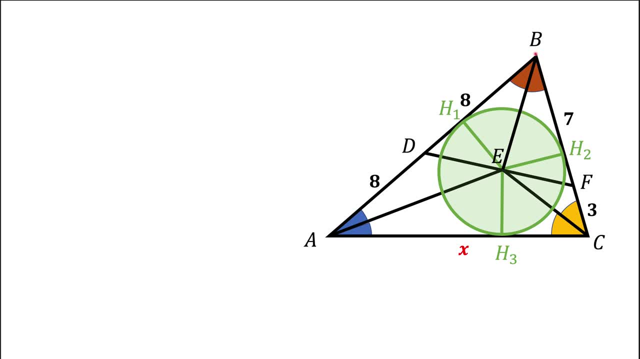 In a similar way, EH2 will be at 90 degrees to BC and EH3 will be at 90 degrees to AC. So let's get rid of the circle. We don't need it anymore, And what we're going to do now is 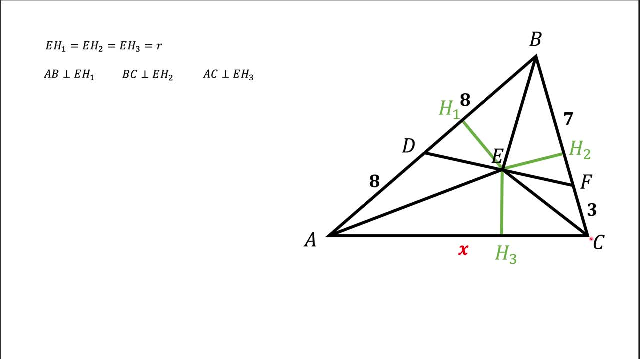 To calculate the area of a big triangle, ABC, And we're going to do it by splitting it into three triangles: That blue, orange and gray. So let's consider triangle AB, the blue triangle. The area of this triangle is the height or altitude. 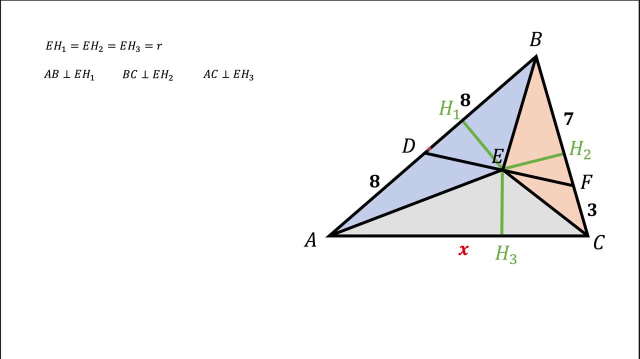 That will be EH1.. Times the side or length of the side of this triangle, So that's going to be the area of triangle AB, and divide it by two. right For the orange triangle it's a half EH2 times BC. 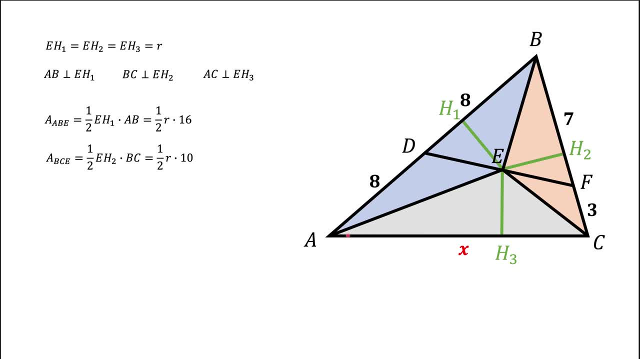 And for the triangle AEC it will be half EH1 times AC. The whole big triangle ABC is the sum of those three triangles, Okay, And we're going to get a formula like this. So there are two unknowns in this formula. 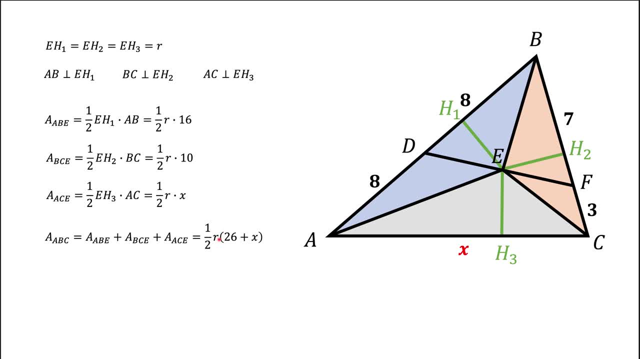 We don't know R, we don't know the radius of the inscribed circle And we don't know X. Okay, So let's move on, And the next thing we're going to do, we're going to calculate the area of the small triangle DBF. 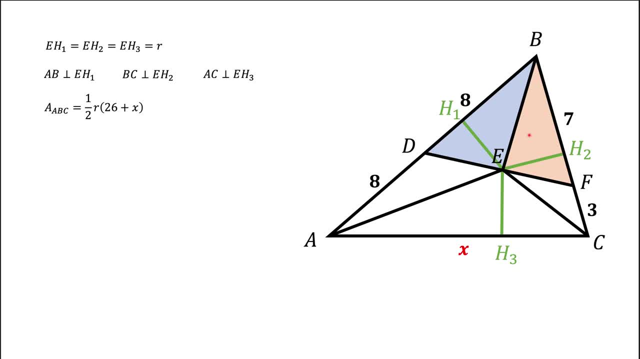 And we're going to split this triangle into two triangles- blue and orange- And calculate the area of each triangle separately. If you look at the blue triangle, its area of it is half EH1 times DB And area of the orange triangle is half EH2 times BF. 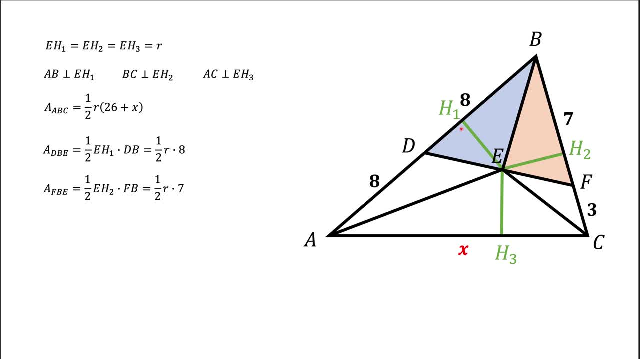 We can find both areas, add them up to get the area of DBF And get a formula like this: Okay, The next thing we're going to do is we get rid of this R, because we're not really interested in R. 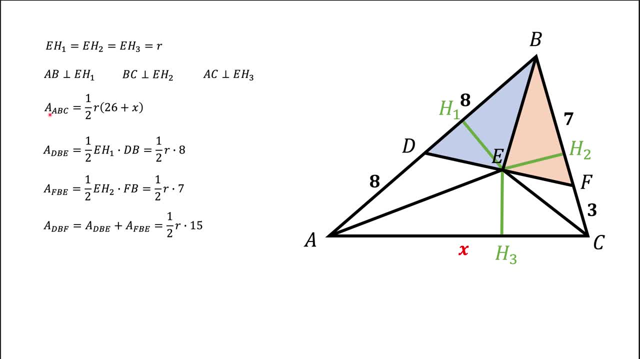 Nobody asked us to find it, So to do this, we're going to just divide the area of one triangle- big triangle ABC, by the area of the smaller triangle, DBF. In this case, we're going to have a relationship that has only X in it. 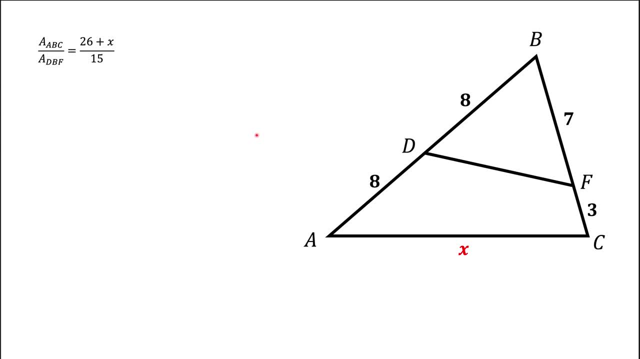 So what we're going to do now is we're going to calculate the area of triangle DBF and triangle ABC using the sides AD, BD, BF and C. Okay, So first we're going to draw a line DG that is parallel to line AC. 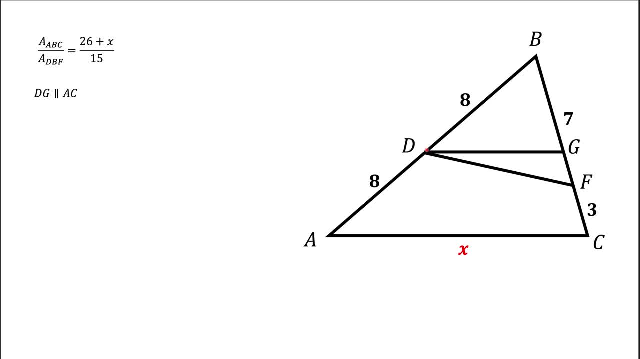 And what we notice is that the triangle at the top DBG is similar to triangle ABC, And that's because, if you look at angle A of the big triangle and angle D of the smaller triangle, those angles are corresponding angles for parallel lines. 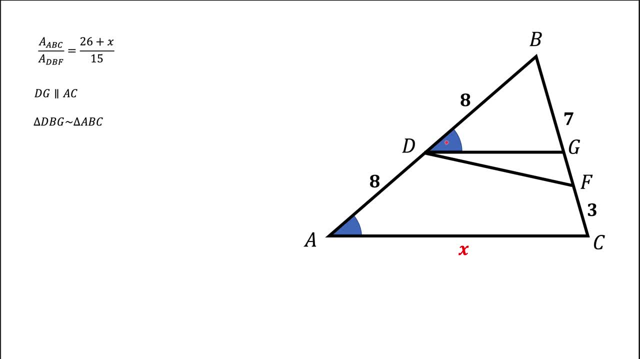 And corresponding angles for parallel lines are congruent. And the second thing is, if you look at angle B, that angle both of these triangles share. I mean. well, in this case that angle is congruent to itself. So we find that these two triangles are similar by two angles. 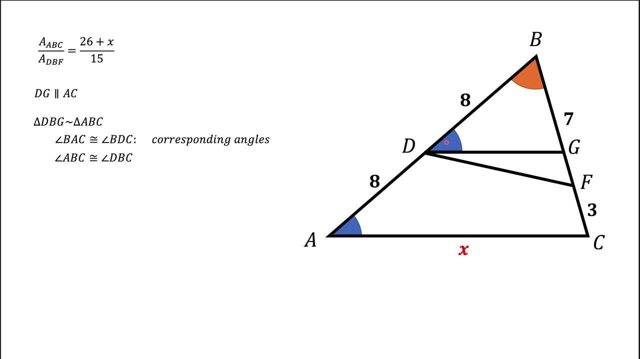 And in similar triangles, the sides are proportional, which means that the ratio of the respective sides should be the same for all sides, And that means that DB divided by AB is the same as DG divided by AC and the same as BG divided by BC. 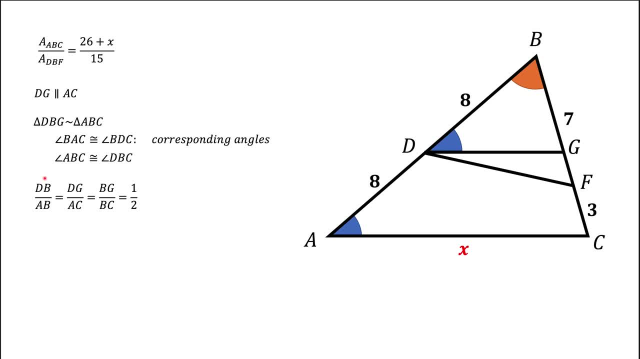 Okay, We know DB over AB. it's half, So we know the ratio of the other sides. The other thing we know about similar triangles is how the areas related to each other, If we know the ratio of the sides of the similar triangles. 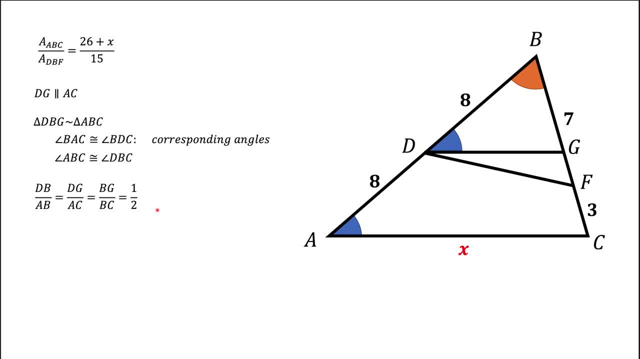 we know that the ratio of the areas of similar triangles should be ratio of the sides squared, And in this case we related the area of the small triangle on the top to the area of the large triangle, ABC. We know from this that BG is half of BC, which make BG 5, and that makes GF 2.. 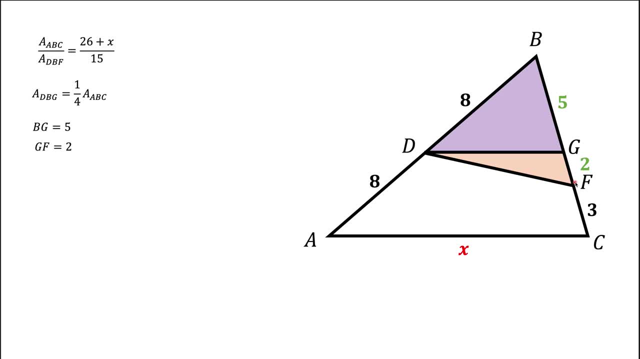 Now we'll look at other triangles. Now we'll look at the top two triangles and we'll try to relate them to each other. Now notice: the purple and orange triangles have the common vertex d, and what we're going to do, we're going to draw an altitude dk from that vertex. 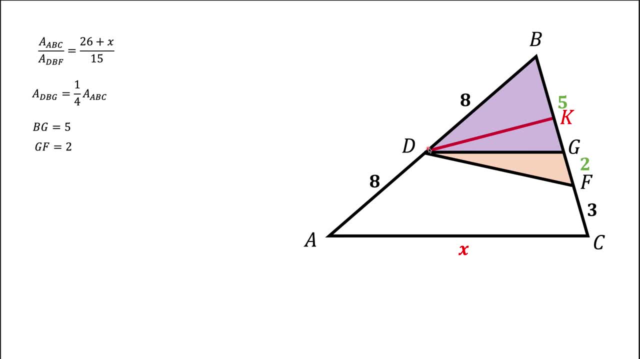 Now notice that altitude is an altitude for both of those triangles. So now, if I want to calculate the area of the purple and the orange triangle, I will do it by taking half of dk times the length of the side. So in case of purple triangle it's going to be bg, and in case of the orange triangle, 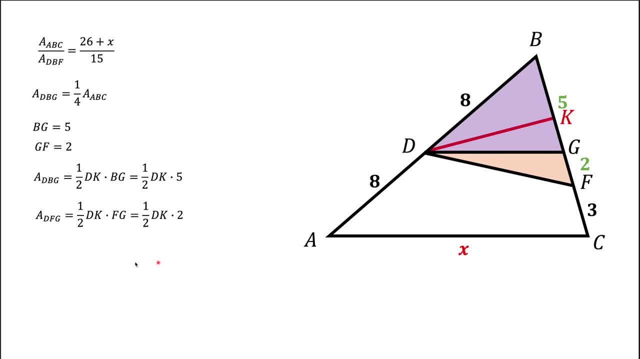 it's going to be fg. And now what I'm going to do? I'm going to divide. I'm going to divide the area of the orange triangle by the area of the purple triangle. In this case, we get rid of dk and we found how the areas of those two triangles are related. 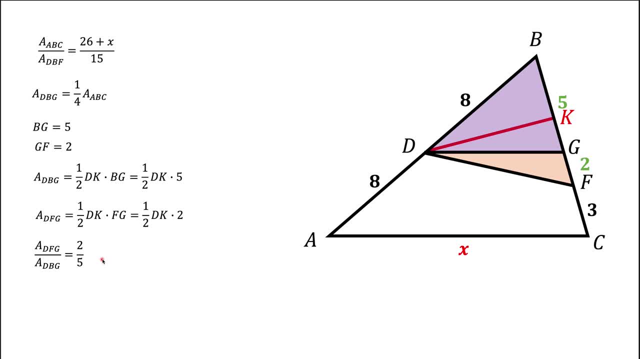 to each other And we can use it to calculate the area of a triangle, dbf, which is sum of areas of these triangles. And we calculate the area of the triangle dbf via the area of the triangle dk. But the next thing is to notice that we know how to relate the area of the triangle dbg. 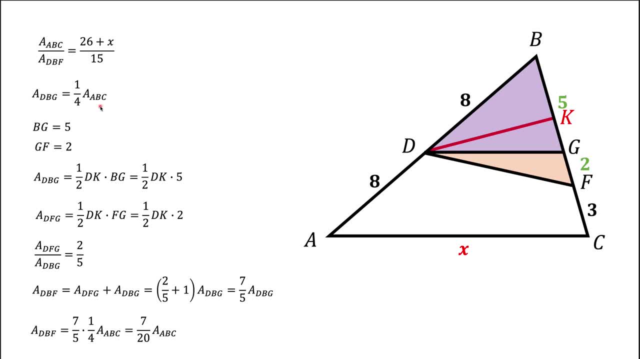 to the area of the triangle abc And this way we relate the area of dbf to the area of the big triangle of abc. We can rewrite it in a different way like this: So we found the ratio of the area of the big triangle to the area of the smaller triangle. 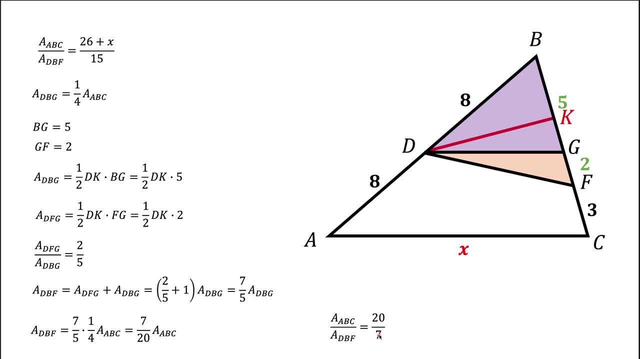 in a different way from the inscribed triangle. So now we have two formulas that are supposed to give us the same result. So from these two formulas we can find x by equating right-hand sides and solving this linear equation by multiplying both sides by 15.. 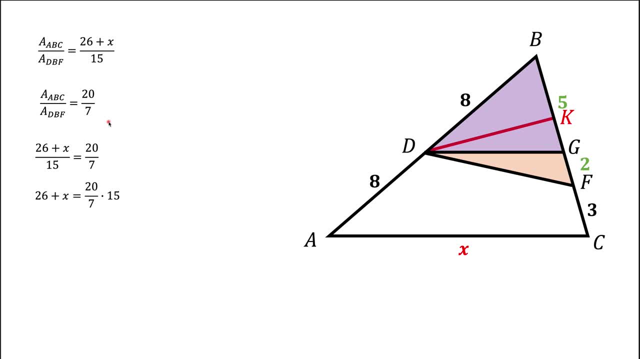 So that's it, Thank you. So we're going to do 15 first, then subtracting 26, and then simplifying the right-hand side to find the final answer.